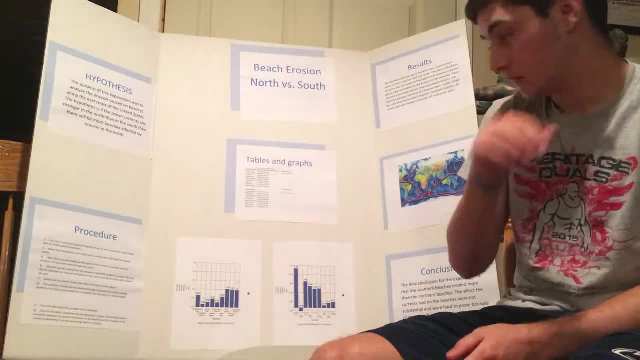 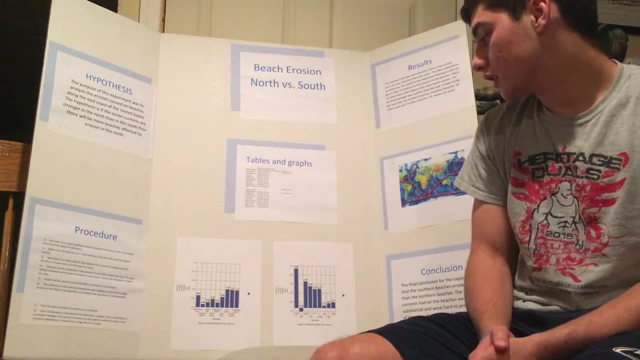 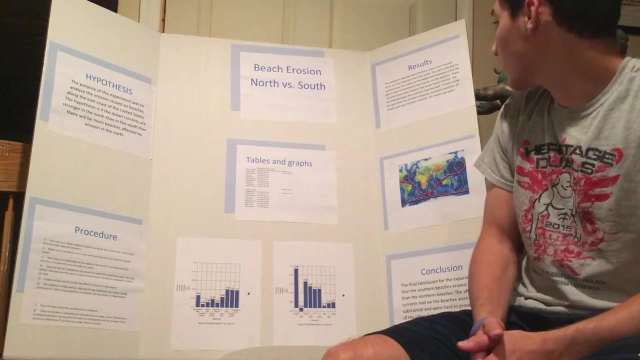 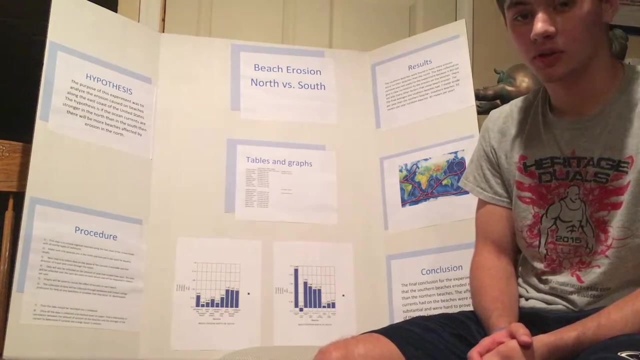 So from there, I collected data on each beach, and the data was in meters per year, and once all of it was collected, I averaged everything out and I found that the southern beaches eroded more than the northern beaches. My results were that the average of the southern beaches was 0.92 meters per year that were eroded. 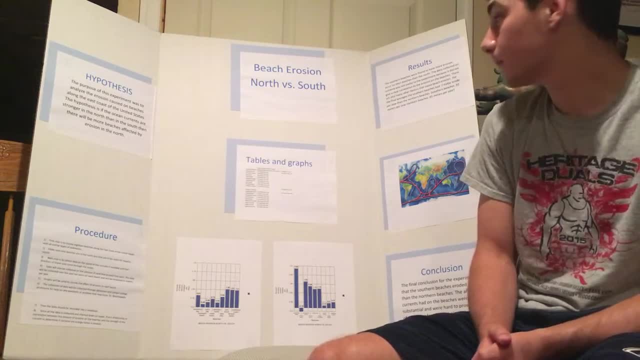 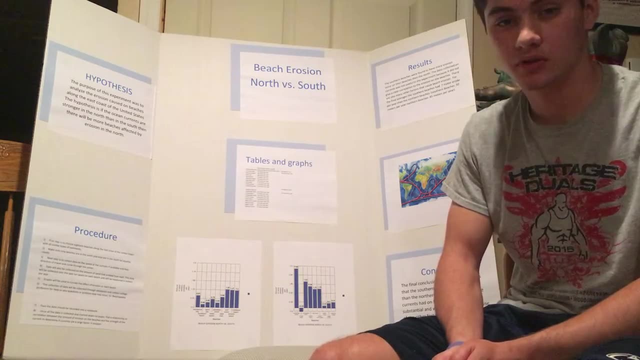 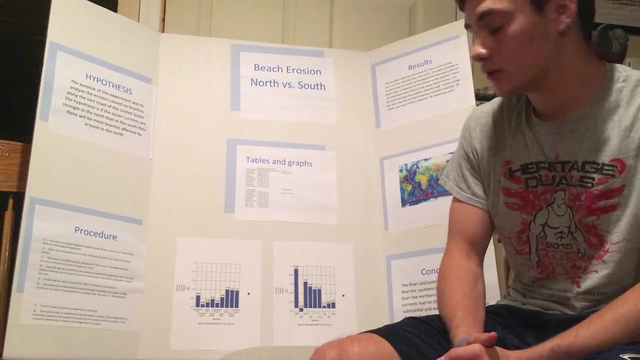 and for the northern beaches it was 0.85 meters per year. So, for my conclusion, I found that my hypothesis was not supported and that the southern beaches eroded more than the northern beaches, and what I found was that currents were not the only factor that involved in erosion. There's a lot more, such as wind, how the beach was laid. 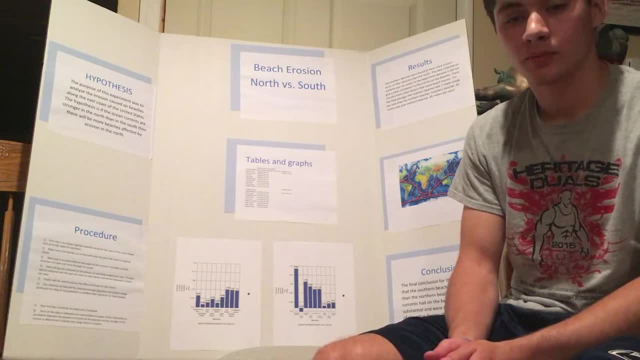 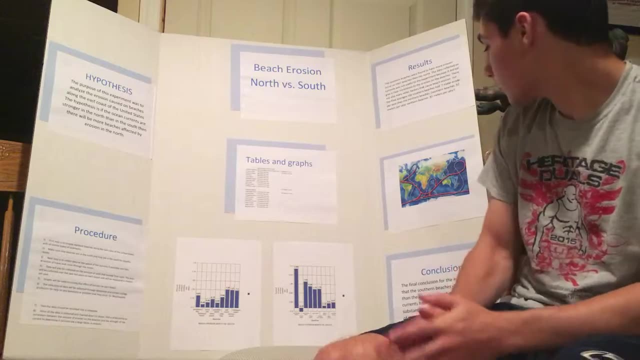 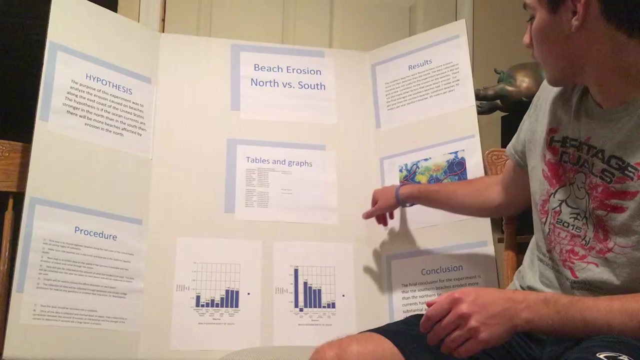 out how the ocean floor was laid out and storms, And what I found was that storms were a huge cause of erosion and if you look at where storms are formed, it's along warm water areas and they go up along the coast and they create hot spots of erosion. 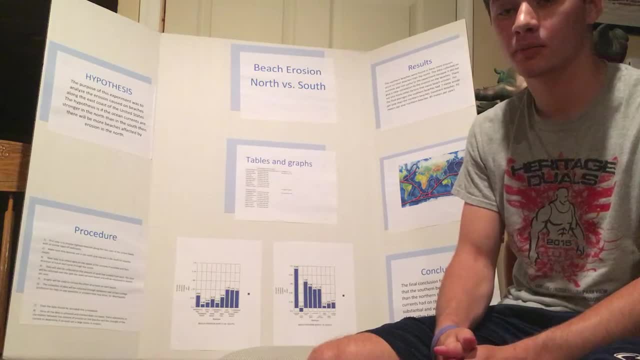 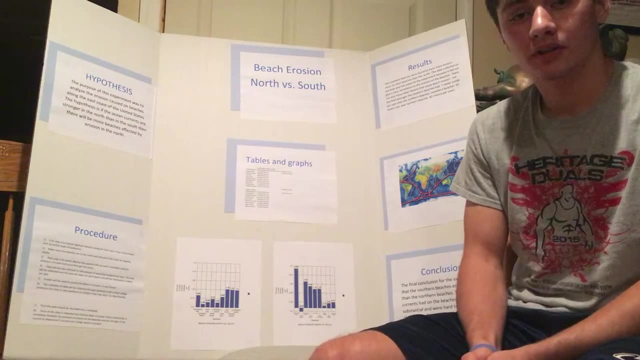 And that's partially why I think my hypothesis is correct. So I think that's why I think my hypothesis is correct. I think my hypothesis is wrong because of the tropical, the tropical storms that are created there And the reason for me picking this topic of beach erosion. 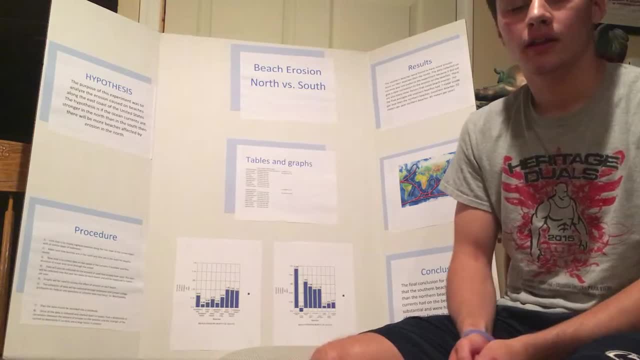 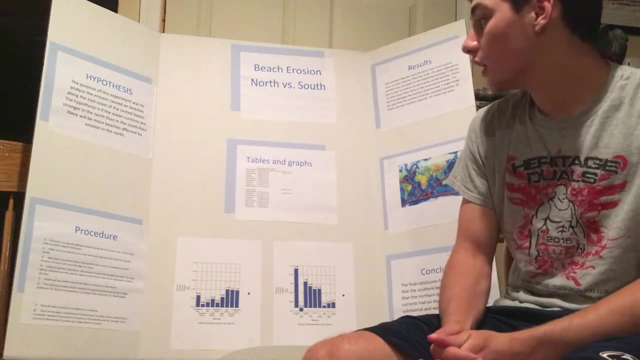 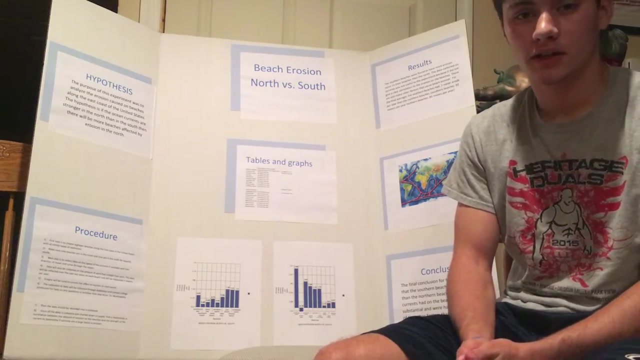 is that I did a project earlier in the year that my teacher gave us and she said: to pick any topic you'd like. so I picked sea turtles. I was interested in them and what I found was that they were endangered of being extinct, and the reason for that is a lot of the 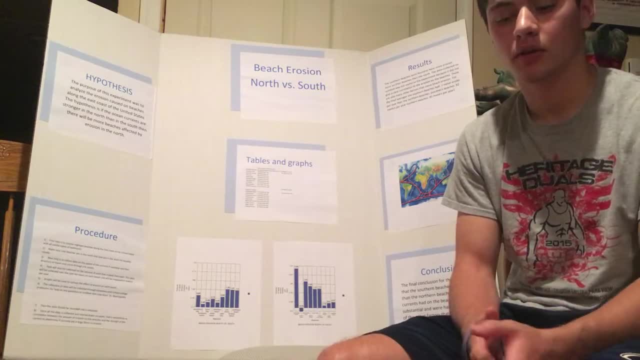 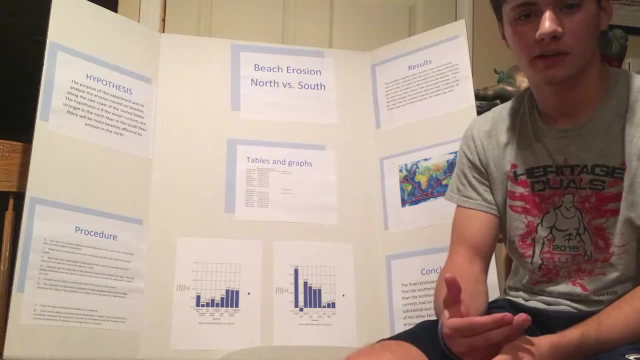 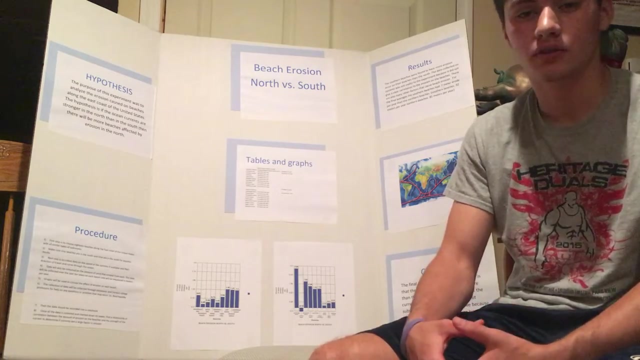 are being eaten on the beaches and when a mom sea turtle comes up to the beaches they lay their eggs and they cover them with sand and they go back to the ocean. but when there's not enough sand on the beaches to cover their eggs, then crabs and seagulls and other predators will come and eat those eggs. 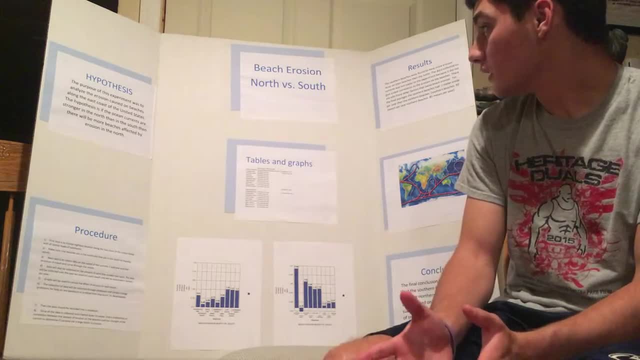 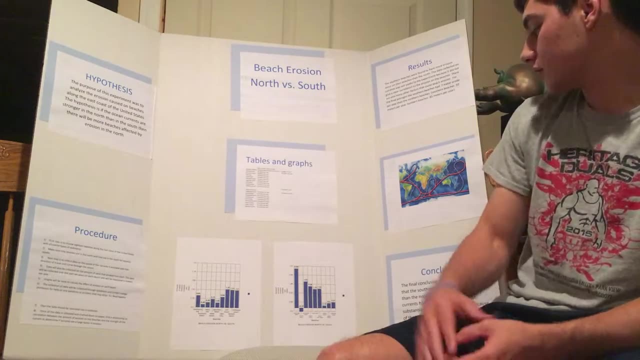 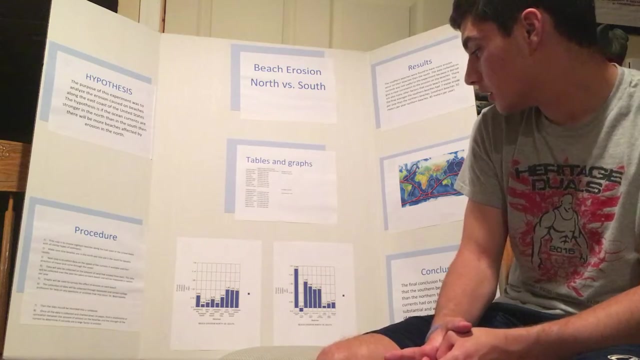 and that's mainly why I wanted to research why these beaches were being eroded. So, as you can see, with the northern beaches, the beaches that I picked were Penobsco Bay, Bucksport Beach, Casco Bay, Reeds Beach, Aberdeen Beach.